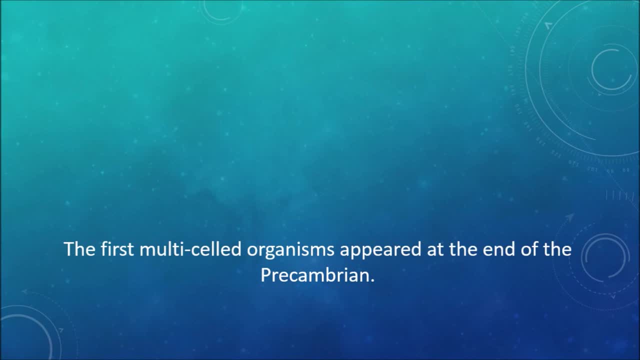 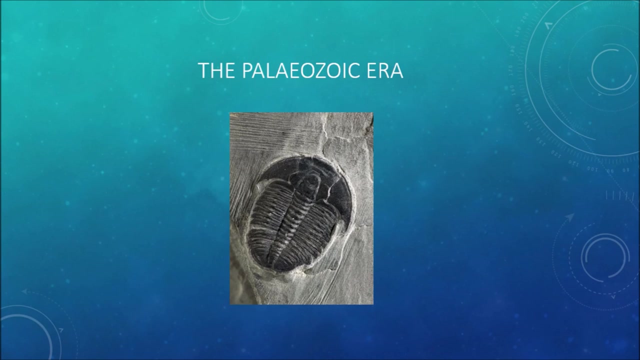 However, a few million years before the Precambrian ended, the first multi-celled creatures appeared. The first animals had soft bodies and looked like nothing alive today. Some of them actually looked more like plants than animals. What do you think this beastie is? The Precambrian ended about 540 million years ago, when we suddenly see animals with shells in the fossil record. This is the beginning of the Paleozoic era. 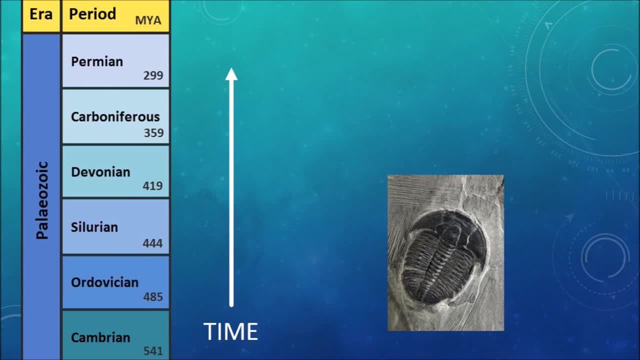 We divide the Paleozoic into six periods. Cambrian, Bordovician, Silurian, Devonian, Carboniferous, Permian. You don't have to remember these names, although it might help you in a quiz one day. 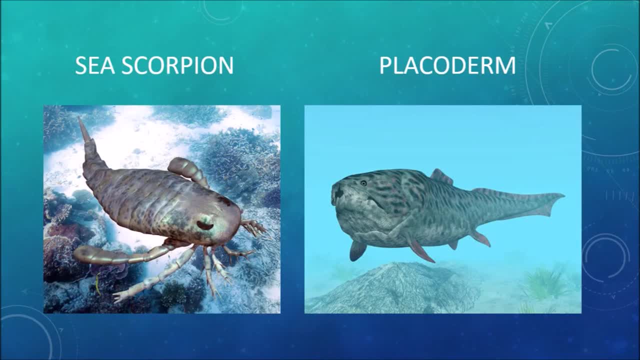 Animals and plants evolved into bizarre and extraordinary forms during this era. As the Paleozoic progressed, an arms race between predators and prey led to the creation of the first backboned animals, our ancestors. They survived terrifying sea scorpions and scissor-toothed fish, eventually clambering onto land on four legs. 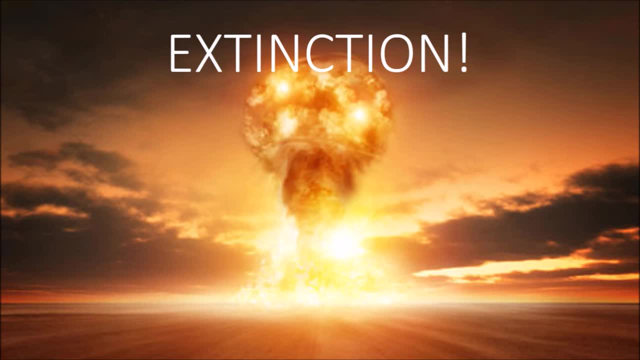 Sadly, it all ended with a mass extinction event at the end of the Permian period. We don't know exactly what happened, but 251 million years ago, 83% of life on Earth was wiped out. Obviously, our ancestors made it through, hiding away in their burrows. 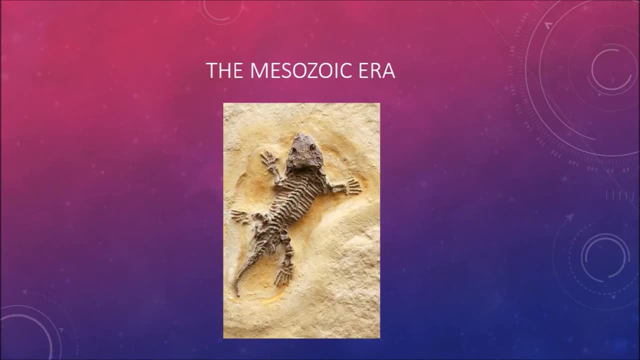 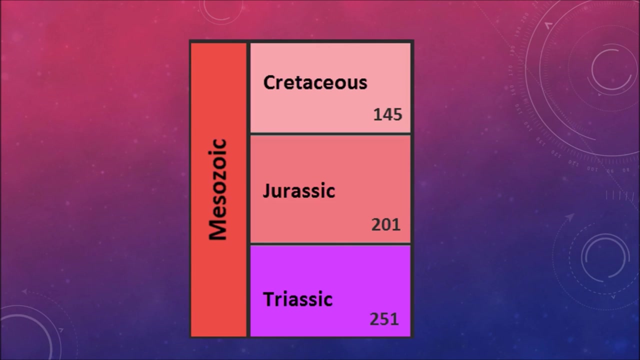 After that catastrophe came the Mesozoic era. This chunk of time is often called the Age of Reptiles, because reptiles were the dominant animals both on land and in the seas. It is divided into three periods, the Triassic, Jurassic, and Cretaceous. 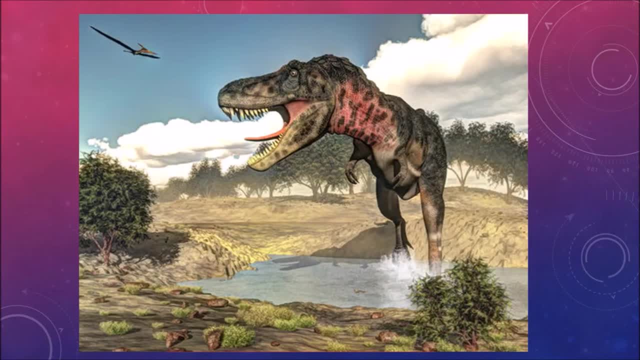 The Mesozoic is the era almost everybody has heard of. This is the time when dinosaurs walked the land. Australia had its fair share of beasties, like this Deer Man, which is one of the most famous animals in the world. The Mesozoic is the era almost everybody has heard of. This is the time when dinosaurs walked the land. Australia had its fair share of beasties, like this Deer Man, which is 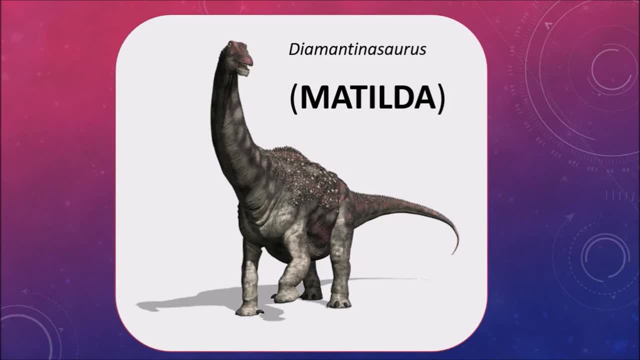 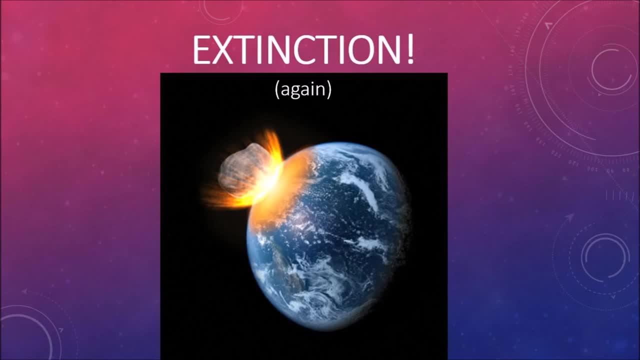 one of the most famous animals in the world. For the ardent, dexterous, and most goblins to enough stars and celestial places, to feed their whole minds at once, deacons won't survive. resonates! 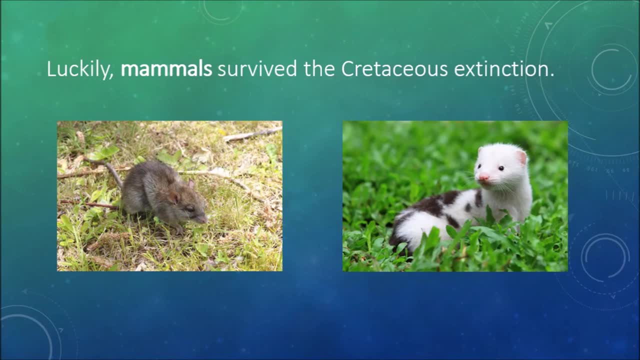 Even though deacons and preocupations began to spread around evolution, with many the 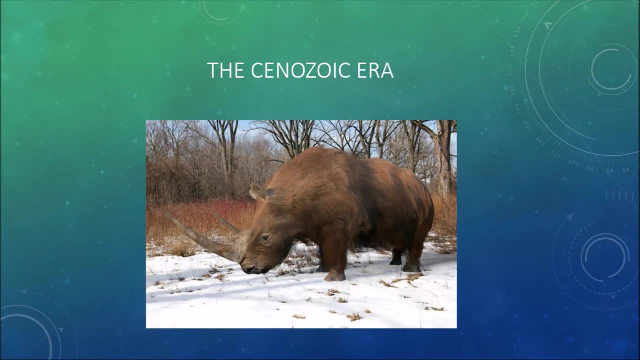 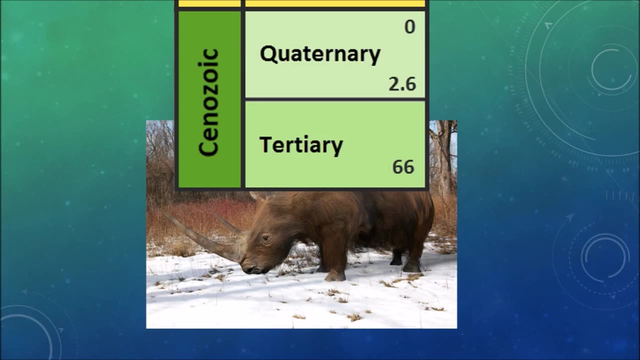 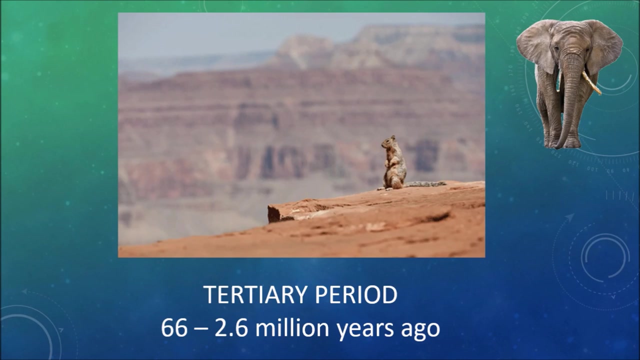 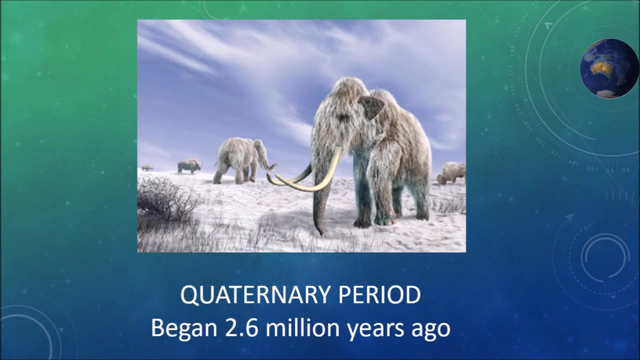 Now we're in the Cenozoic era, the time since the Cretaceous catastrophe. Scientists divide the Cenozoic into two main periods, the Tertiary and the Caternary. In the Tertiary, mammals finally had room to grow. They started out as timid burrowers, no bigger than a cat, but before long they had diversified, with elephants stomping around on land, and whales cruising the oceans. We are living in the Caternary period, which started 2.6 million years ago. This span of time is significant because it covers the evolution of humanity. 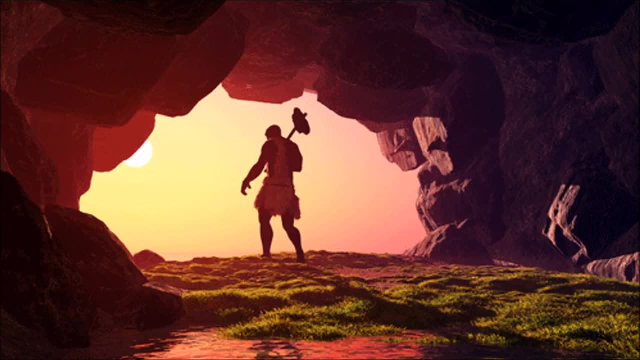 Through a long cycle of ice ages, our human ancestors endured, and ultimately spread from Africa to every corner of the earth. 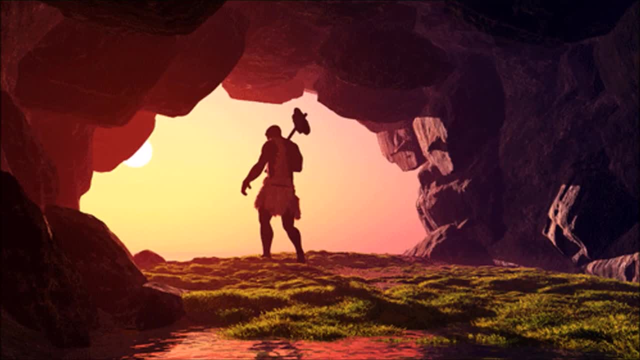 We think the first Aboriginal Australians set foot on this land a few tens of thousands of years ago. 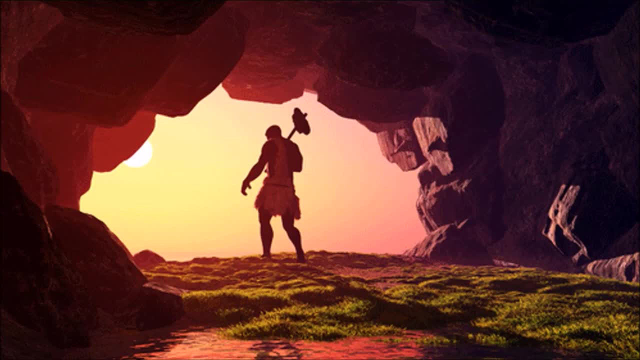 They were joined much later by Europeans. And that is where I think we are. 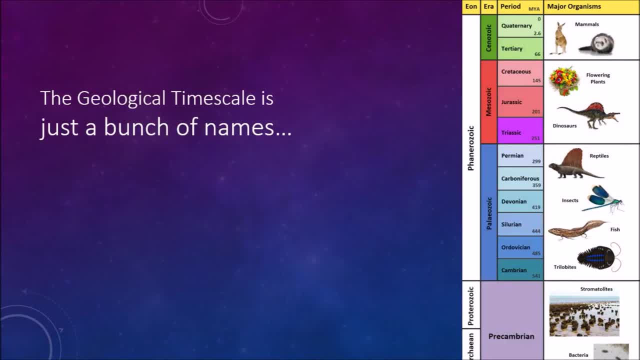 All we see on the geological timescale is a series of names, Cambrian, Ordovician, Silurian and so on. 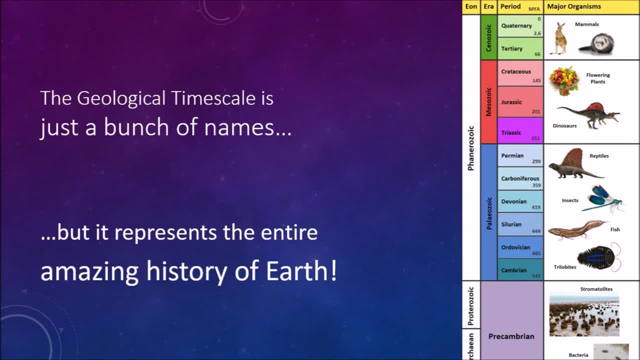 But when you look at where those names came from and what they represent, you end up seeing back in time. 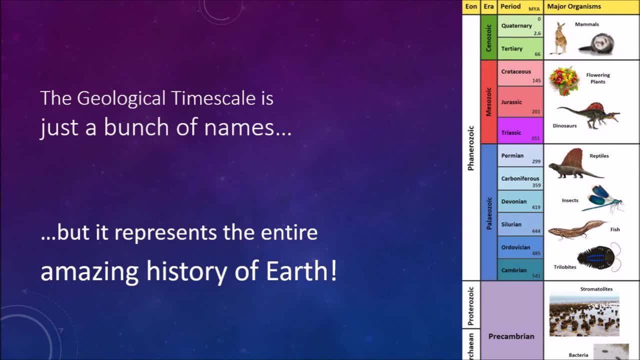 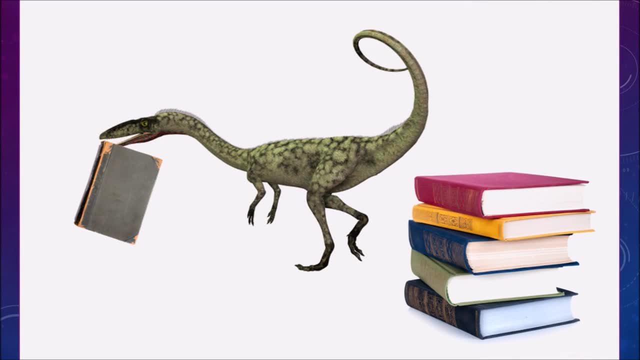 The history of the earth is dramatic and utterly mind-boggling. If you'd like to know more about the timescale and the amazing history it represents, there are many good books on the subject. 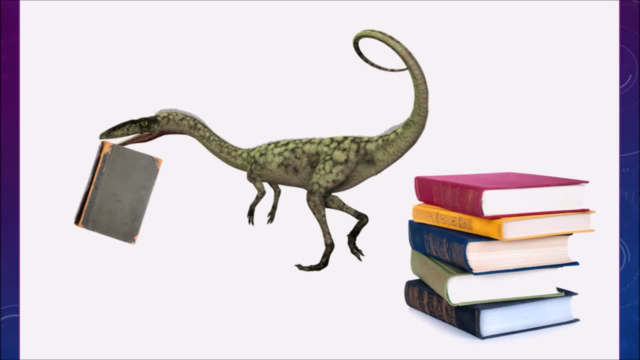 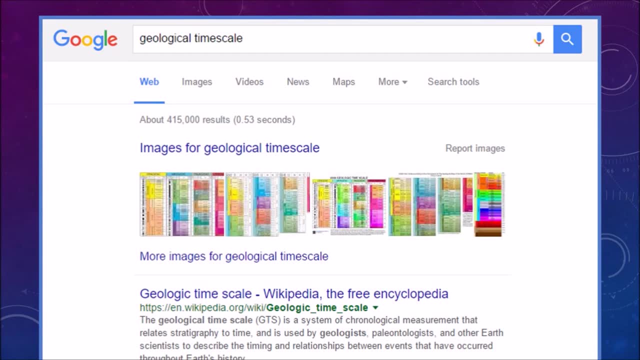 Just have a look in the non-fiction section in your local library. You can also find plenty of resources online, but please ask your parents' permission before searching on Google. 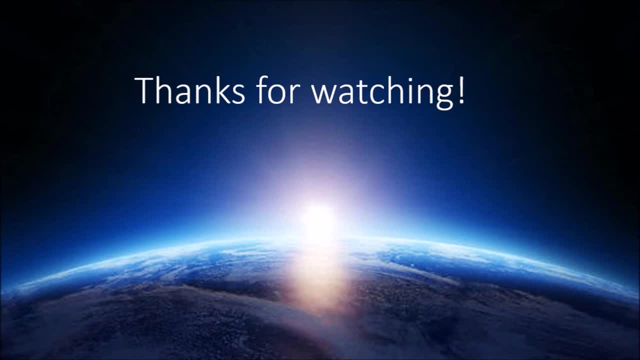 That's all for now, thank you for watching, and good luck!